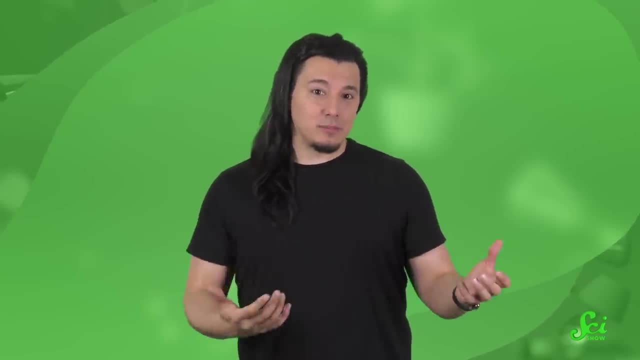 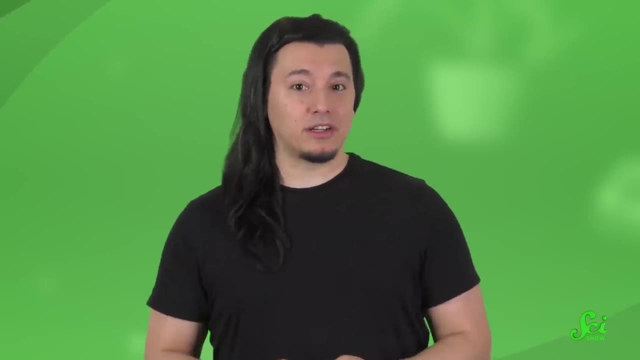 whether they are tiny single-celled plants or meters long like kelp. They've also served as food for thought for some scientists, inspiring them to use algae to improve upon many of our everyday products, From sunscreen to oil. let's take a look at five products. 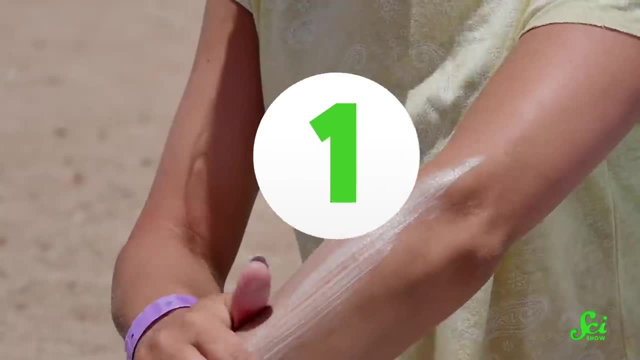 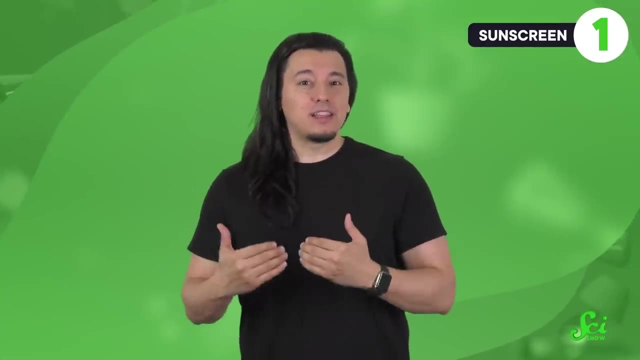 that are in development that use algae as a muse. Humans aren't the only ones that need to use sunscreen as protection from the sun. Even those that rely on the sun for their food need to protect themselves from it. sometimes, Algae spend a lot of their time soaking up ultraviolet rays. 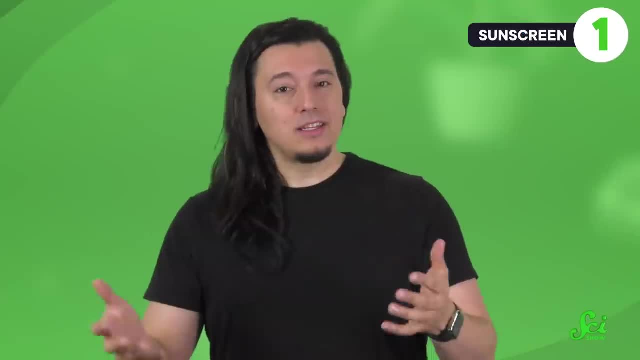 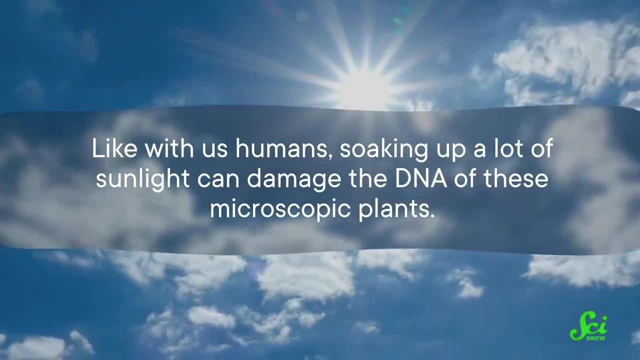 because the sun is what helps drive photosynthesis. Without it, these tiny plants wouldn't be able to create their food. But too much of something isn't great either. Like with us humans, soaking up a lot of sunlight can damage the DNA of these microscopic plants. 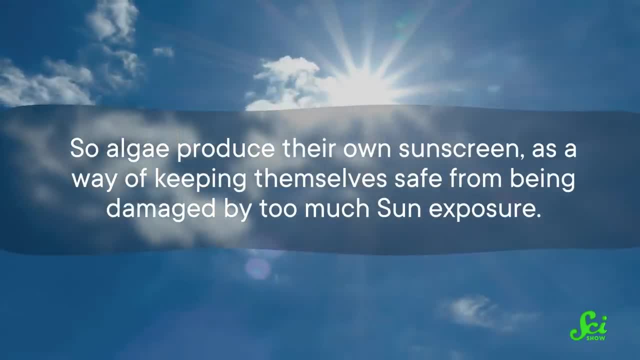 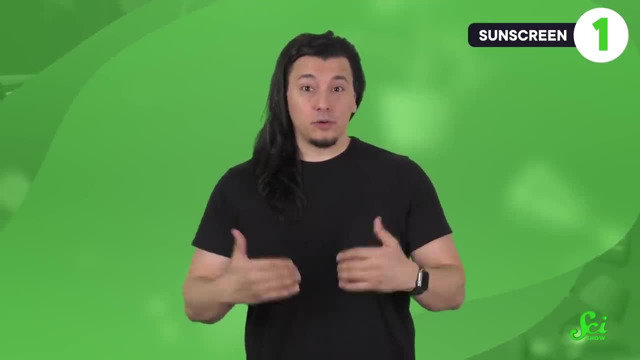 So algae produce their own sunscreen as a way of keeping themselves safe from being damaged by too much sun exposure, And researchers are drawing inspiration from the chemicals that algae produce to shield themselves in order to make a better, less damaging alternative to oxybenzone. 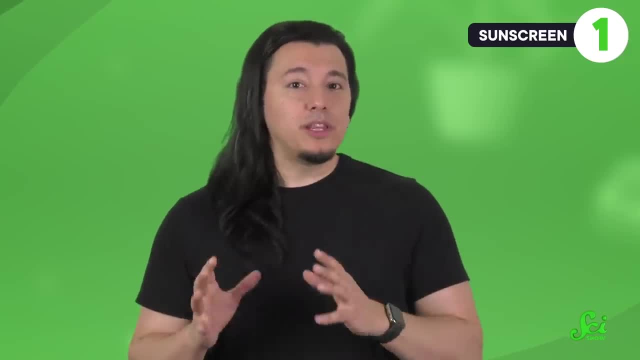 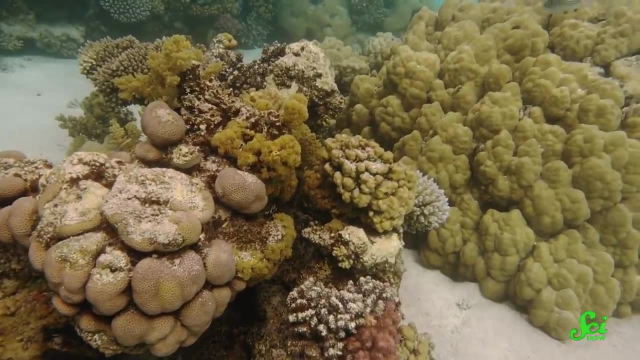 a common active ingredient found in sunscreen. Oxybenzone works really well as a sun protectant, but it can be bad news for the environment. In ocean ecosystems, it's been shown to cause stress to corals, making them more susceptible to bleaching and causing irreparable damage to their DNA. 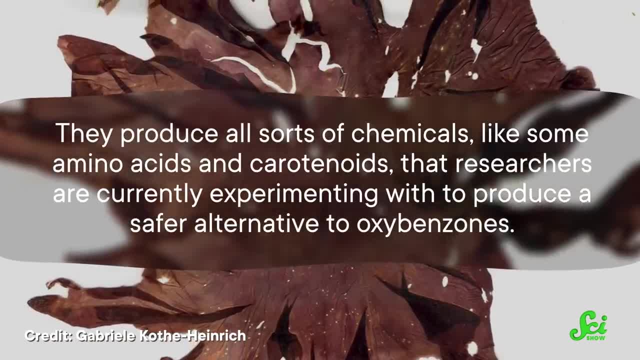 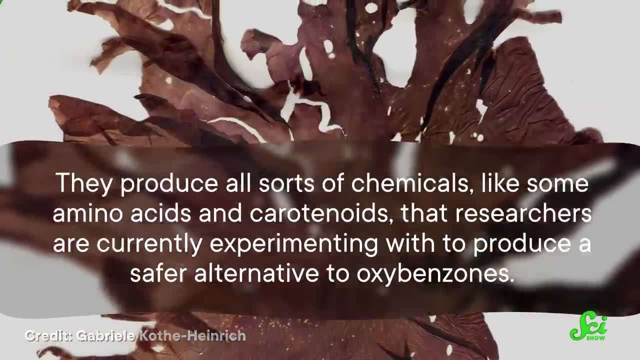 But algae can provide an alternative. They produce all sorts of chemicals, like some amino acids and carotenoids that researchers are currently experimenting with to produce a safer alternative to oxybenzones. Not only that, but they are also pretty good at absorbing UV rays. 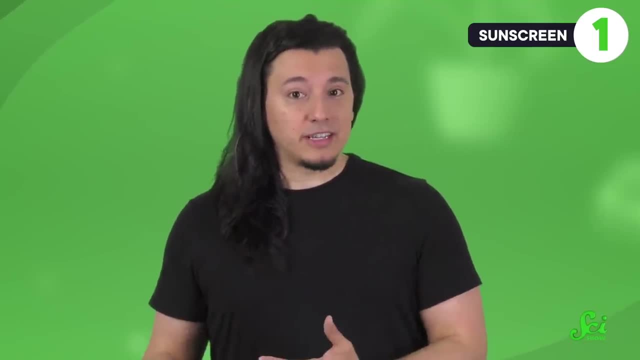 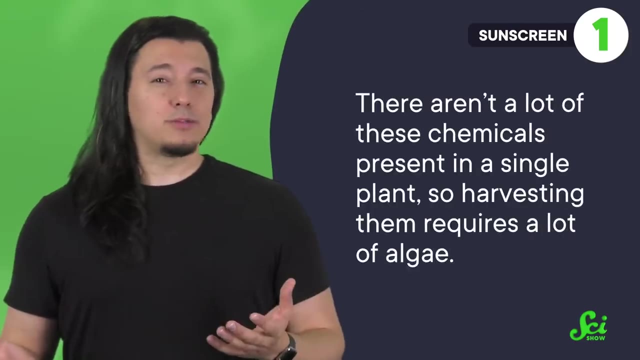 and some may even prevent DNA damage instead of causing it. But there are still some hoops to jump through before sunscreens made with compounds derived from algae make it on the commercial market. Like there aren't a lot of chemicals present in a single plant, 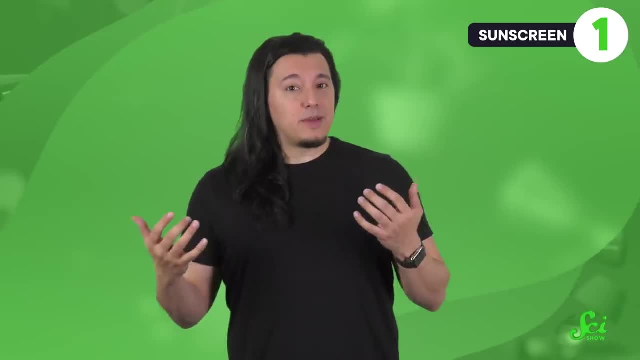 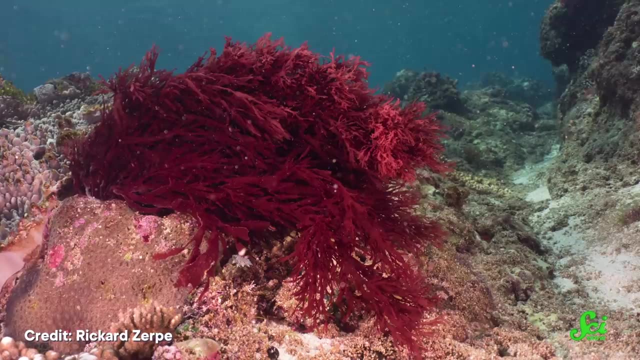 so harvesting them requires a lot of algae. Not only does this make it expensive, but it could also negatively impact algal populations. Researchers are aware that the harvest has to be done in a sustainable way, where the benefits outweigh the costs. Or maybe it's just the case that the 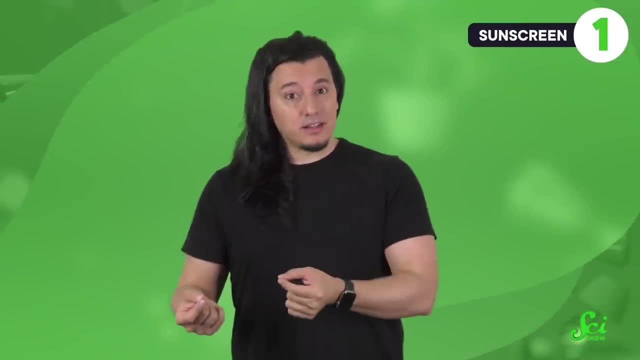 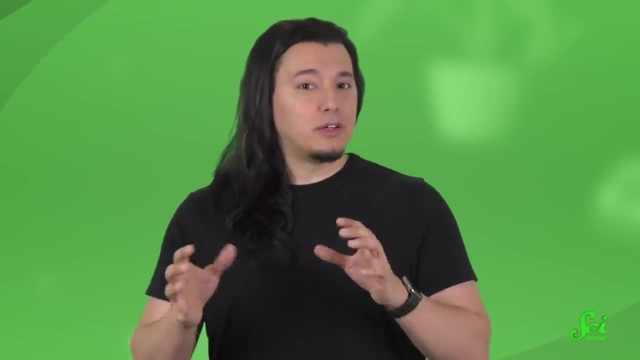 need to isolate which chemical is best and attempt to make it synthetically. Still, algae-inspired sunscreens have a lot of promise, and it wouldn't be too surprising to see them adorning shelves in the next few years, once all the kinks have been worked out. 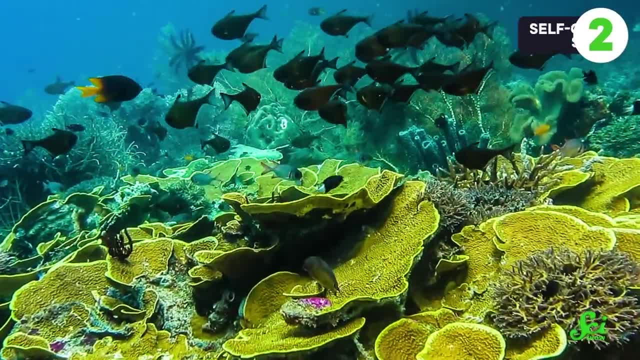 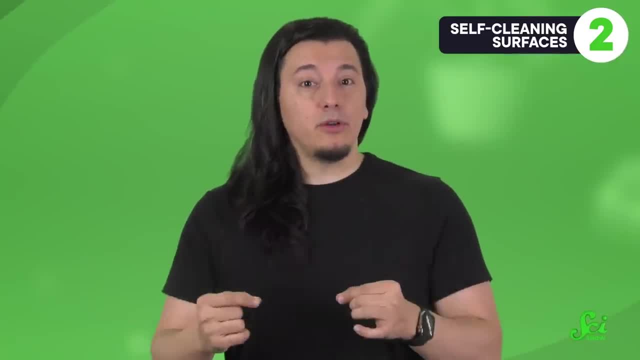 Not only do algae produce their own sunscreens, but they also work to keep themselves from being infected by the billions of bacteria that live in the ocean. Some algal species have the super-cool ability to produce a chemical that keeps the bacteria from forming a biofilm, a thin layer of interconnected cells on the algae. 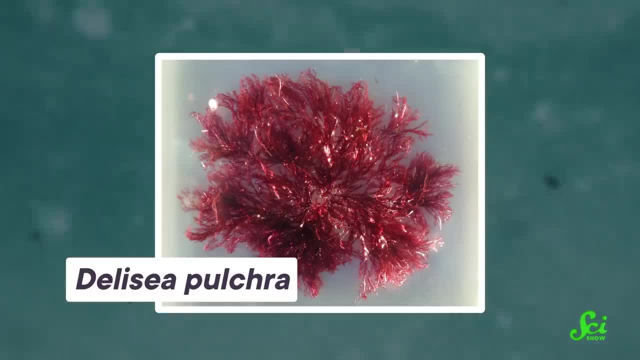 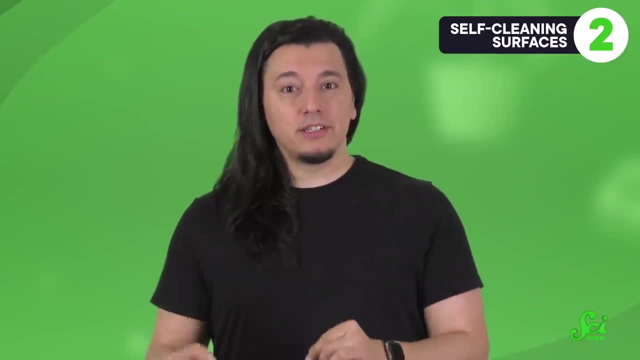 Researchers have found that the red algae known as Delicia pulchra doesn't have biofilms coating its surface like other algae species. That's because it produces a substance that disrupts individual bacterial cells' ability to talk to each other, And if they can't communicate with each other, 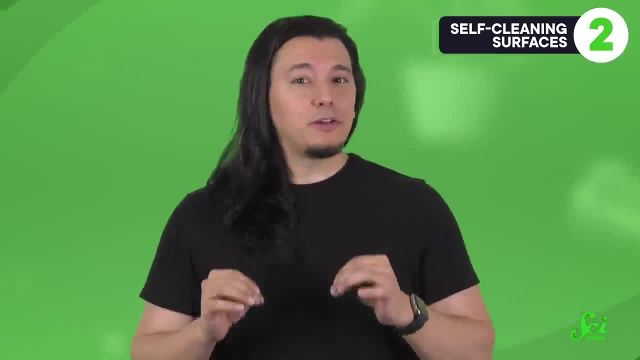 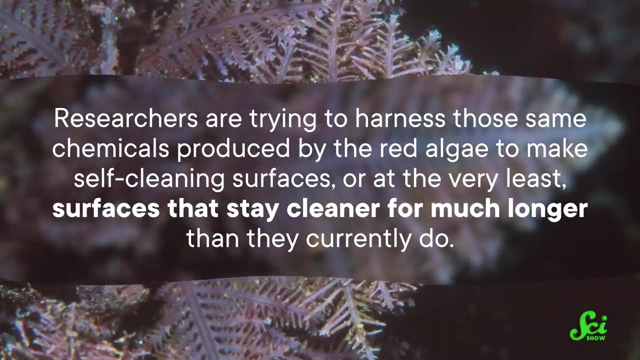 they can't coordinate and form a biofilm on the algae. This particular chemical also keeps bacteria from producing an enzyme that breaks down certain types of antibiotics. Now researchers are trying to harness those same chemicals produced by the red algae to make self-cleaning surfaces, or at the very least, surfaces that stay cleaner for much longer. 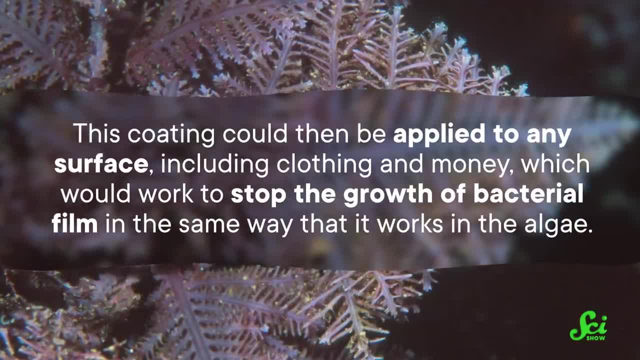 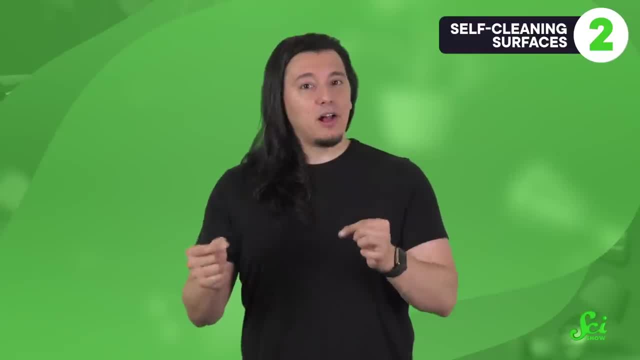 than they currently do. This coating could then be applied to any surface, including clothing and money, which would work to stop the growth of bacterial film in the same way that it works in the algae, And the company has already reported that in trials. 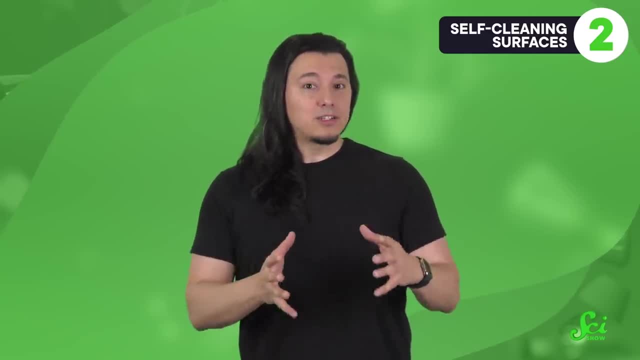 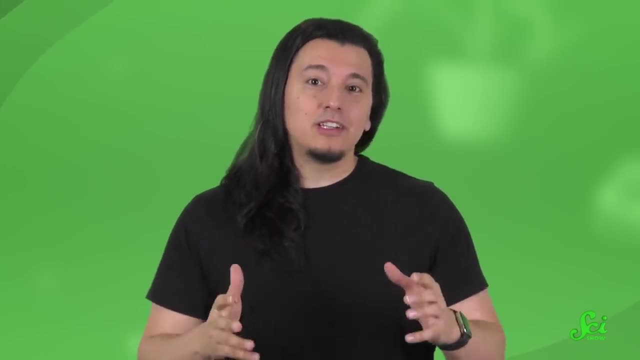 this chemical appears to work not only on bacteria but also fungi. While we don't have self-cleaning money yet, it's definitely in the works, thanks to the incredible resiliency of an unassuming plant. Another super-useful thing that algae produce are oils and fatty acids. 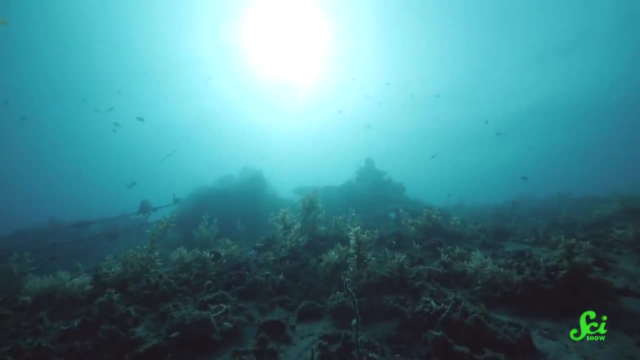 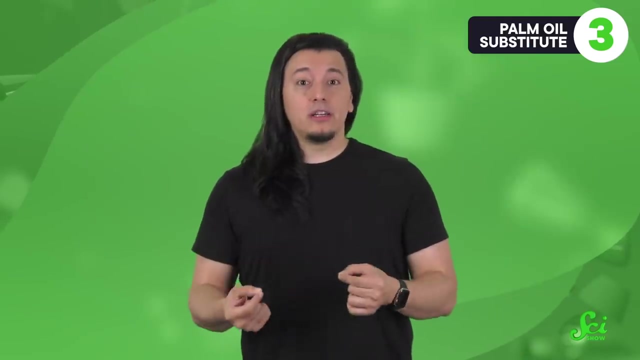 These fats are produced by the algae during the photosynthesis but accumulate in the individual cells. when the algae are stressed out, like when nutrients become scarce, They store these fats up in order to have an energy reserve to tap into until the stressful conditions pass. 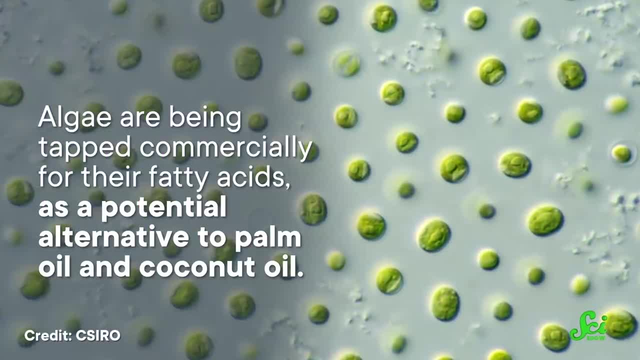 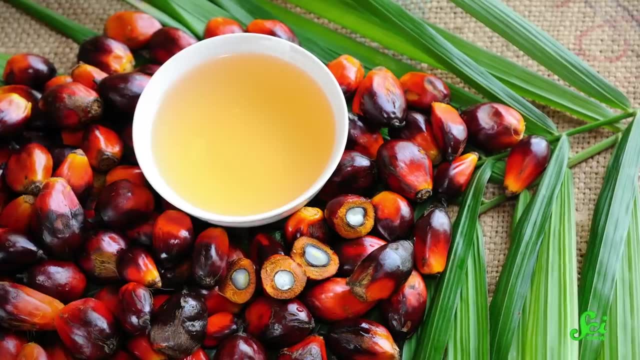 And now algae are being tapped commercially for their fatty acids as a potential alternative to palm oil and coconut oil. Palm oil is used in a lot of everyday products, but it's a particularly controversial source of oil. The harvesting process is driving deforestation and causing the extinction. 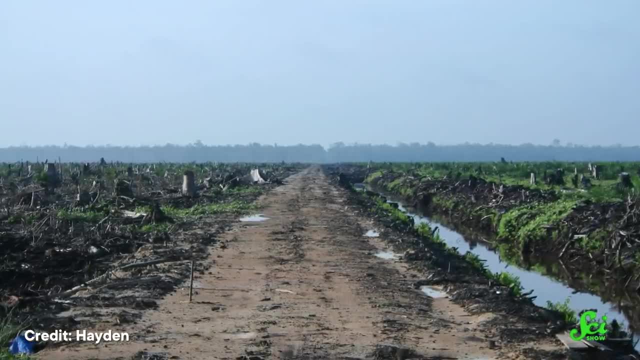 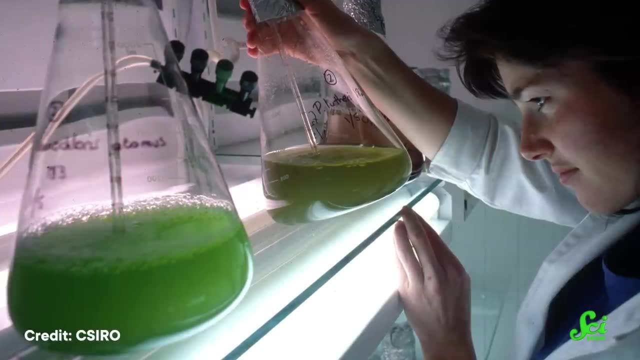 of several species in the forest where the oil gets lost. So finding a non-controversial alternative is necessary to protect these vital ecosystems, And that alternative might just be algae, For one algae don't take up as much space, and harvesting them for their fatty acids doesn't lead to deforestation like palm oil. 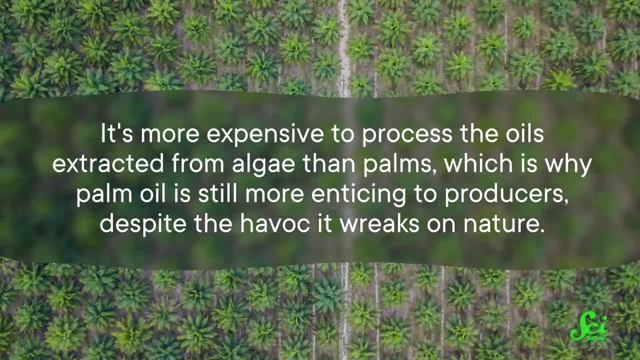 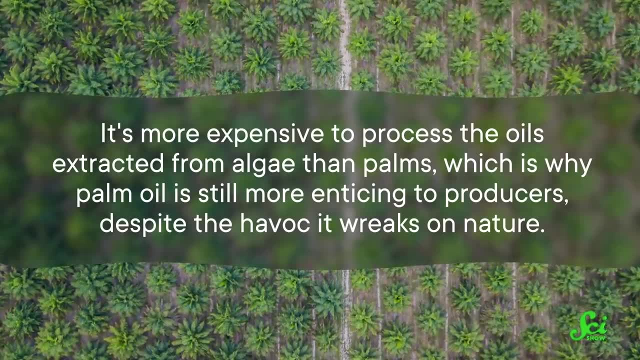 Currently, the major hurdle is the expense. It's more expensive to process the oils extracted from algae than palms, which is why palm oil is still more enticing to producers, despite the havoc it wreaks on nature. But with more research, trials and better technology, 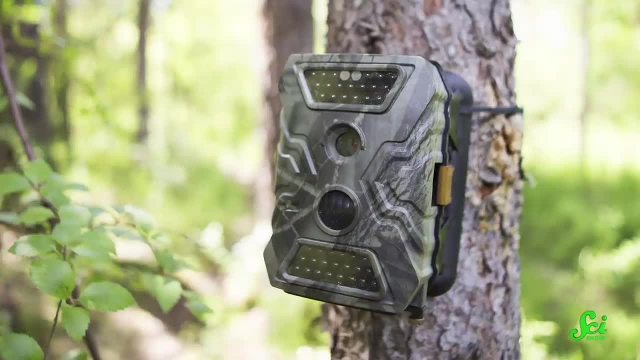 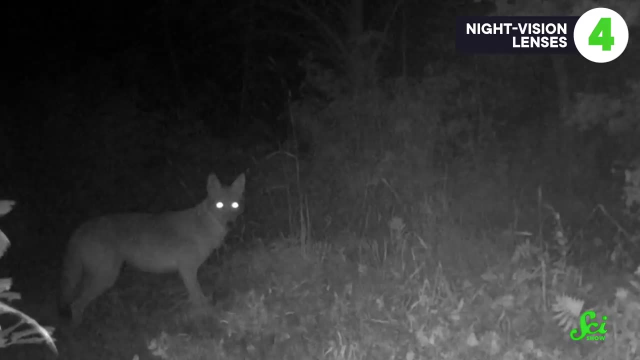 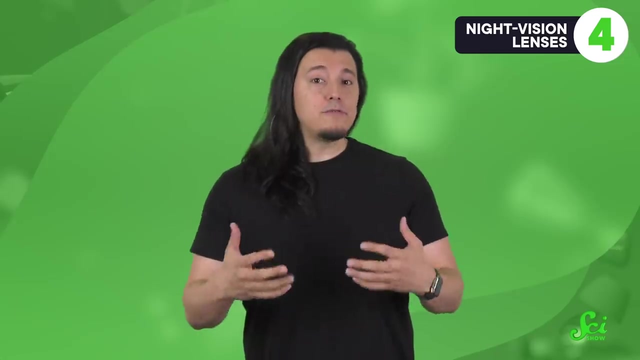 researchers could make progress. Another, less conventional use of these oils produced by algae are lenses, Specifically night vision goggle lenses. Cameras that work in the dark have a lot of uses, everything from the military to security systems, to wildlife tracking cameras. But current infrared night vision lenses are pretty expensive. 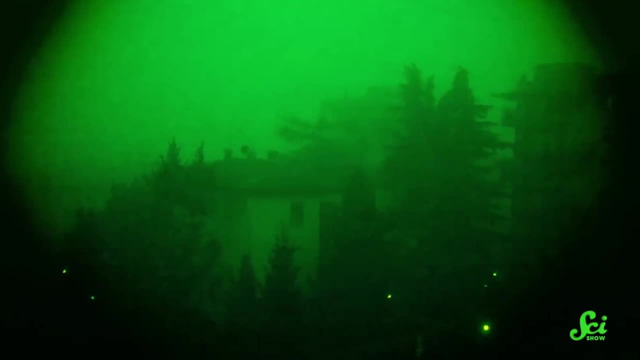 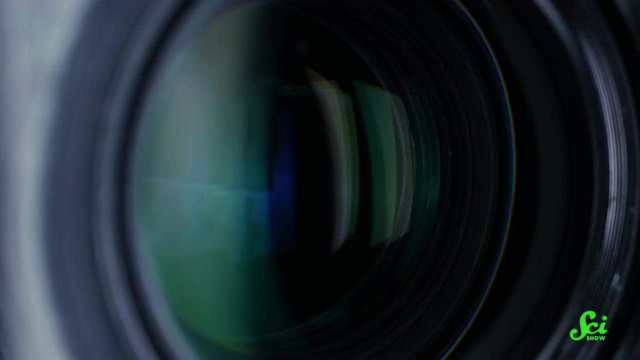 and the images they produce aren't the best quality. And the main reason they're expensive is because when you switch to night vision, you need to also change the focus of the lens, Kind of like changing lenses in a regular camera to focus on something that's far out or close up. 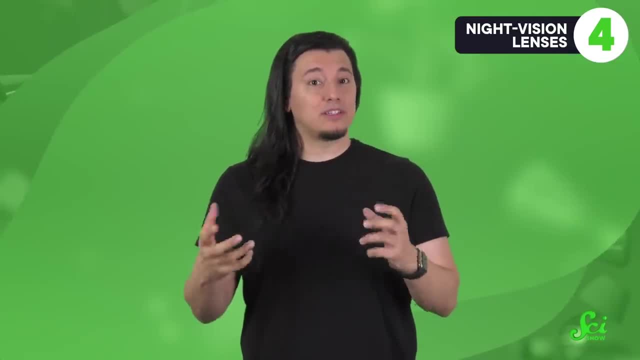 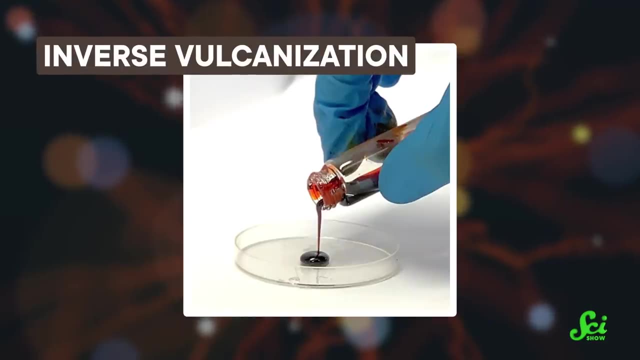 Plus, they need to be able to hold their shape as their focus is changed. This ability is what makes them so expensive. But to make lenses with algal oils you need a process known as inverse vulcanization, which is a pretty cool process in and of itself. 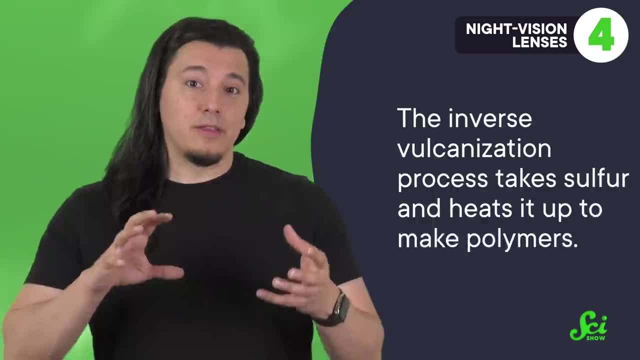 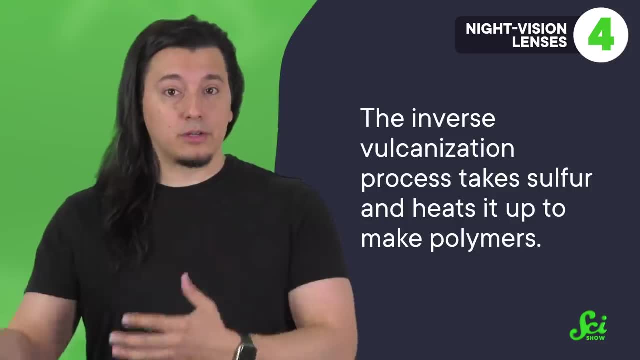 Normally, polymers are made from petroleum-based products, but the inverse vulcanization process avoids petroleum products altogether. It takes sulfur, an unwanted byproduct of refining petroleum, and heats it up to make polymers. And because the algal oils are high in potassium, 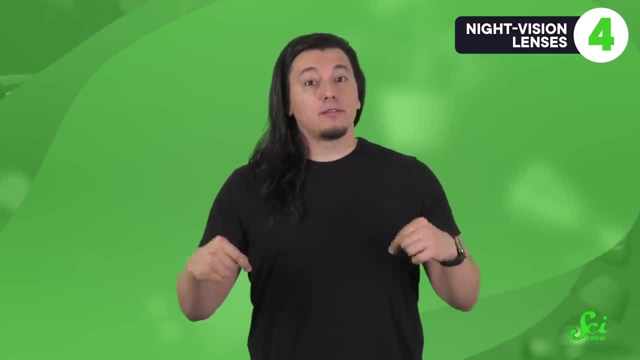 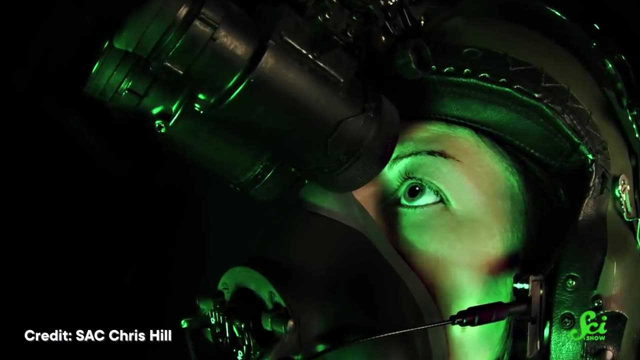 These oils are made up of long chains of carbon atoms. Their length helps make the newly formed polymer stable and stretchy. Because night vision cameras are widely used in so many situations, there is a high demand for their lenses to be made from commonly available. 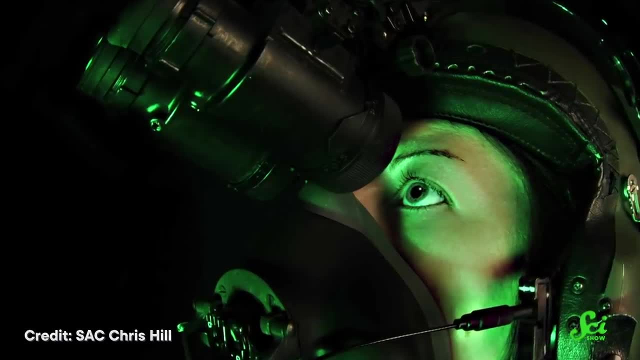 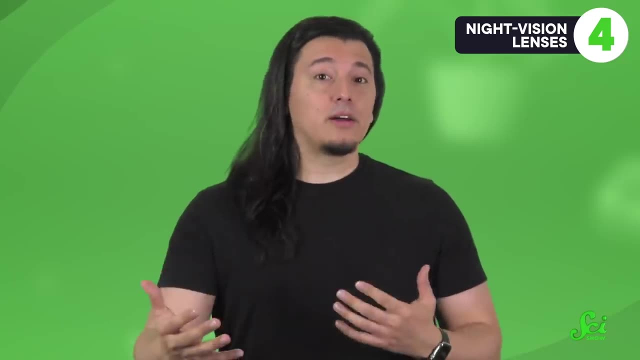 cheap materials that can provide a better user experience, So using a more flexible product can drop the cost of the lens while still hanging on to its ability to focus, And harnessing products naturally produced by algae may be just the trick to attaining lower-cost flexible lenses. 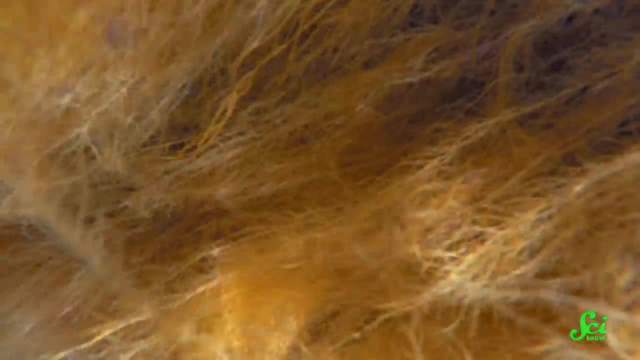 So far we've learned that algae have a lot of tricks up their… cells. They can produce their own sunscreen, antibiotics and fats. Oh, and they can also make their own food- plus at least half of the oxygen on the planet. 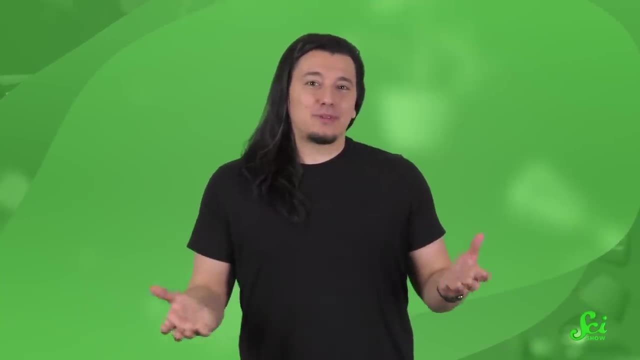 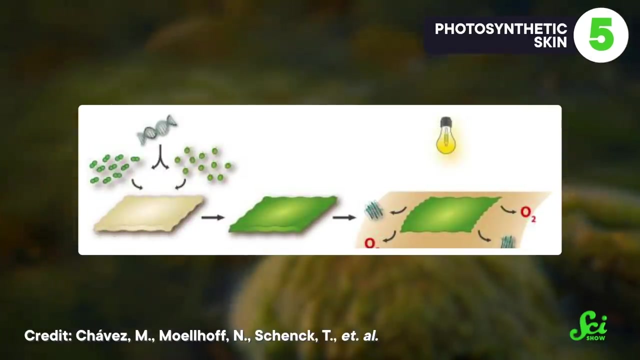 That's some amazing skills for anything, let alone a plant. When did you last make your own food and the air that you need to breathe? But it doesn't end there. Researchers are looking to harness the photosynthetic abilities of algae to create photosynthetic skin grafts. 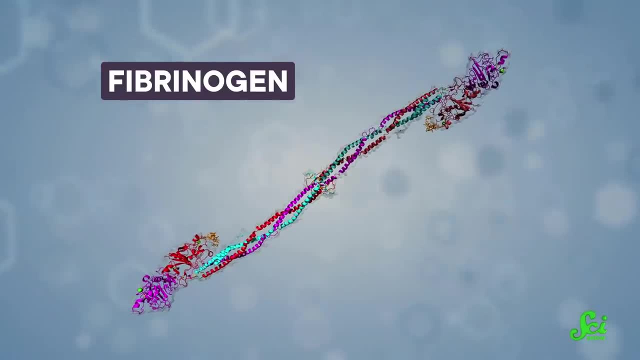 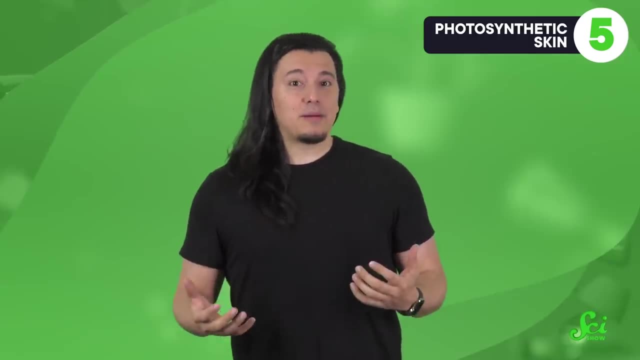 They're combining algae with fibrinogen, a collagen-like protein. This combination creates a material with the photosynthetic qualities of algae and the strength of the protein And, thanks to the plant part of the material, this product not only uses photosynthesis to feed itself. 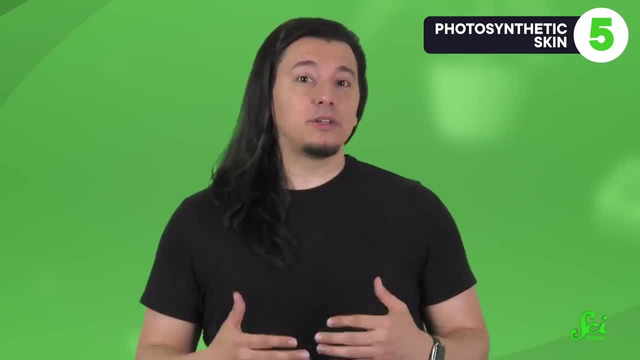 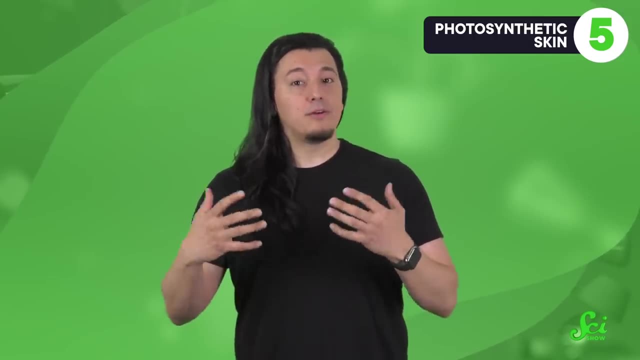 it produces oxygen in the process, Which is exactly why researchers hope to be able to use this material for a skin graft. They see these types of grafts as a big improvement over regular skin grafts because they can produce oxygen. This means that the photosynthetic graft could be applied to tissues. 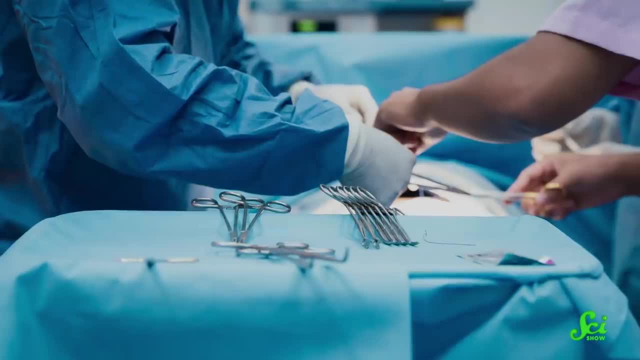 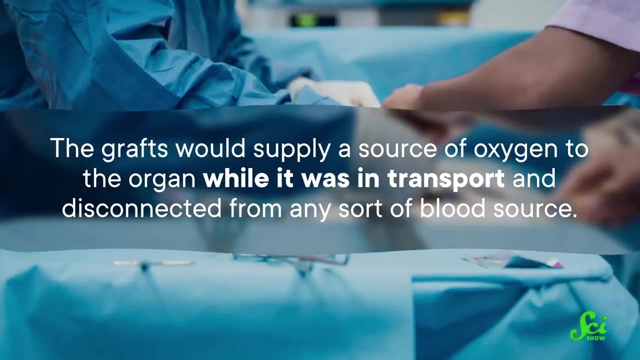 even if there was a lack of proper blood flow to that area. These types of grafts could also be used to keep organs alive during organ transplantation. They're also known as transplant procedures, because they would supply a source of oxygen to the organ while it was in transport and disconnected from any sort of blood source. 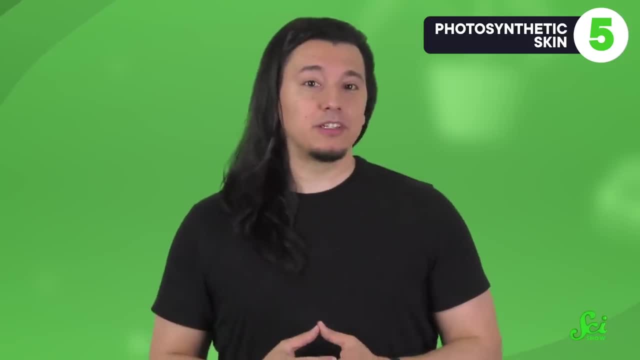 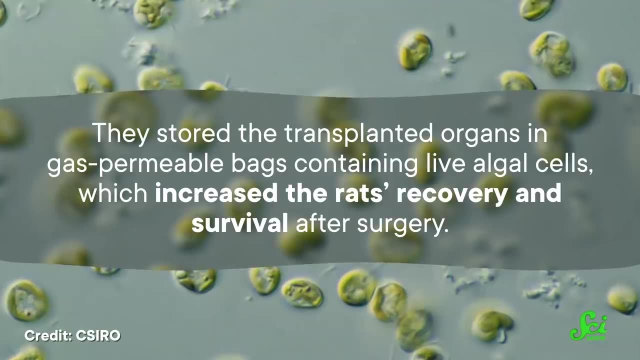 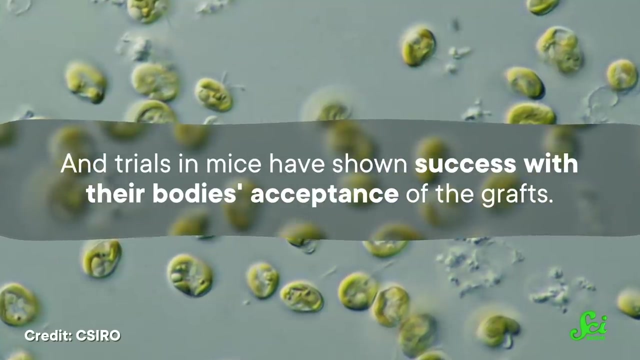 And researchers have already found some success with a rudimentary version of this, at least in rats. They stored the transplanted organs in gas-permeable bags containing live algal cells, which increased the rats' recovery and survival after surgery, And trials in mice have shown success with their bodies' acceptance of the grafts. 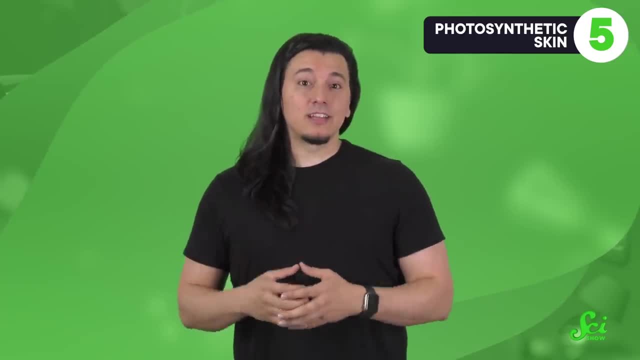 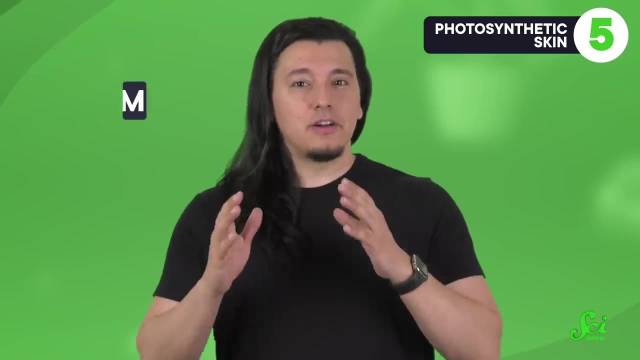 Not only did the mice immune systems not reject the algal cells, but the part-plant, part-animal tissues began to bond better, a process often referred to as a chimera. Also, a very recent trial in humans has found that these types of grafts 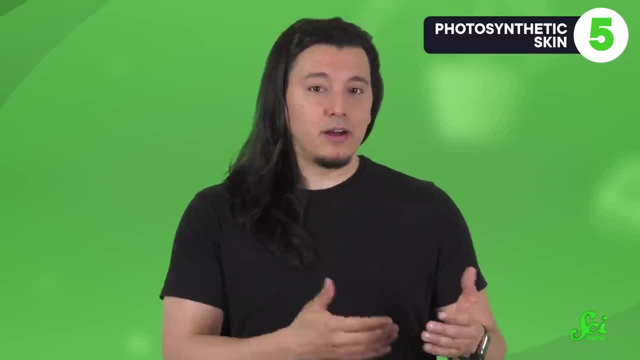 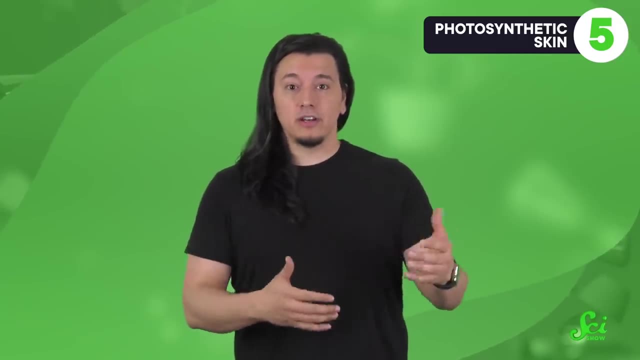 have promise in that the patients' bodies didn't reject them. although that's as far as researchers have taken it so far, There's a lot more work to be done to see if these types of grafts are going to be more beneficial in the long run over more traditional skin grafts. 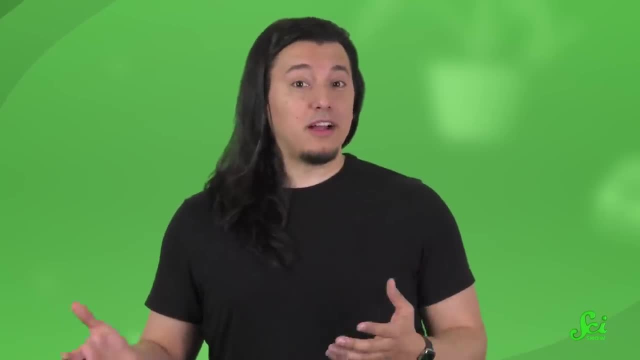 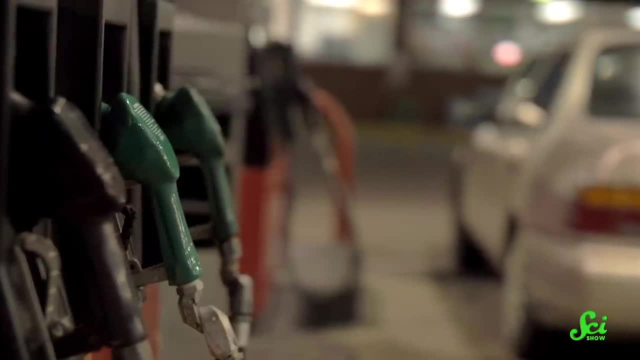 It's a plant that has been used for a long time. It's a plant that has been used for a long time. It's a plant that has been used for a long time And there's already been a flurry of work around creating biofuels. 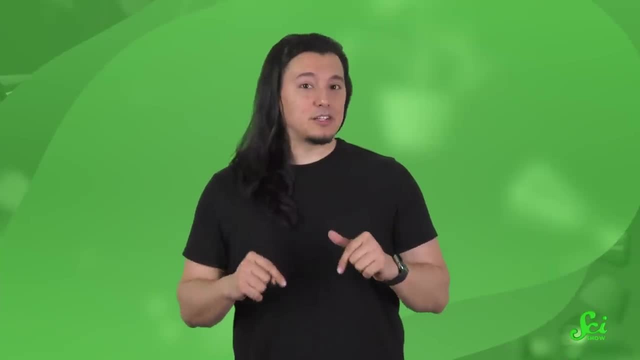 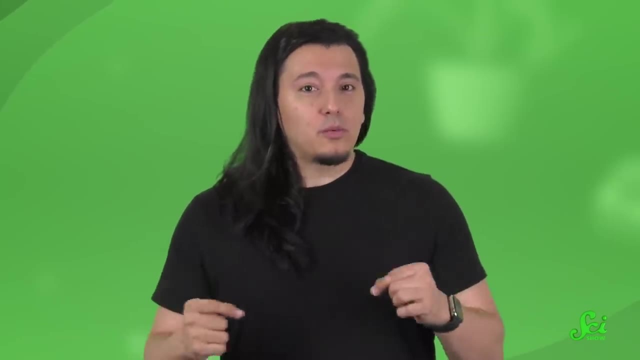 from the oils produced by algae, But I think it's safe to say that these algae-inspired products are taking things to the next level, From sunscreen to photosynthetic skin grafts and everything in between, with a little more work and a lot of innovation. 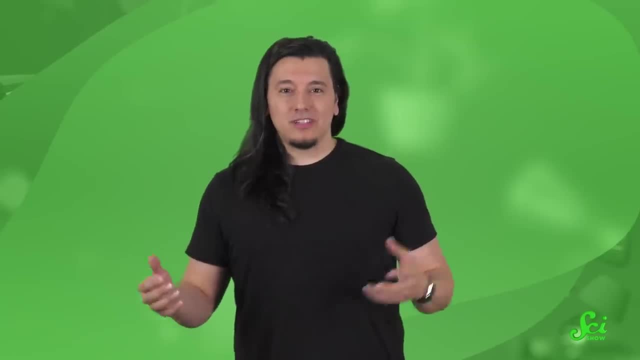 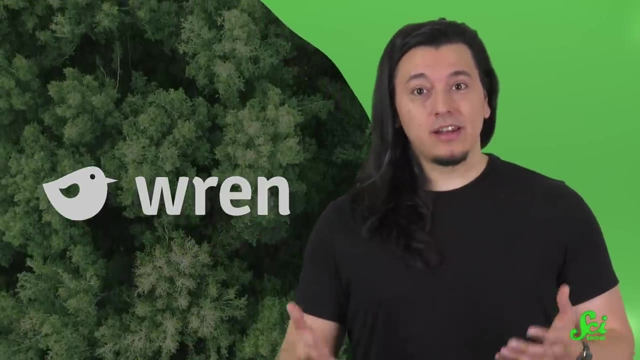 Beyonce's song may soon need a new verse. Who runs the world? It's algae. Algae runs the world, But something that shouldn't run the world is carbon emissions, And today's sponsor, REN, can help with just that.